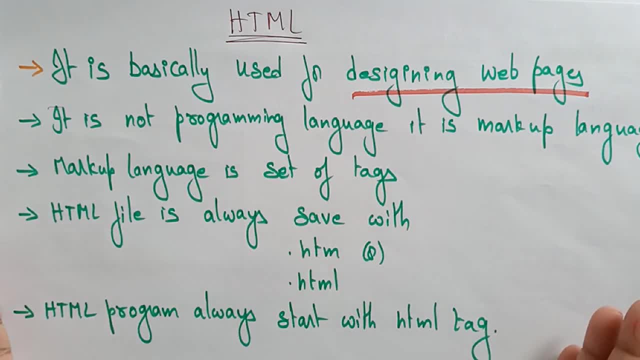 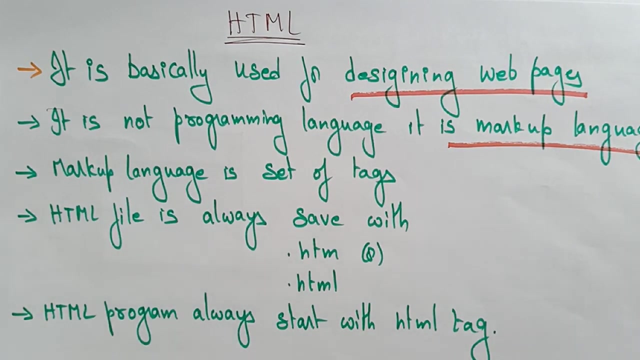 you a HTML in a theoretical part. If you want the practical concept of HTML, just go through that, my videos which are present in education for you. The HTML which I showed everything in practical- Okay, I executed in the browser. Now let's see HTML. it is not a programming language, It is a markup language. So this you have to be remember that it's not a programming languages like C, C++, Java. So it's not like that, It's just simple a markup language. It's not a 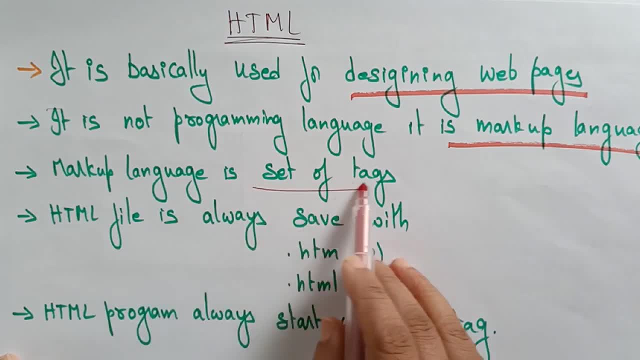 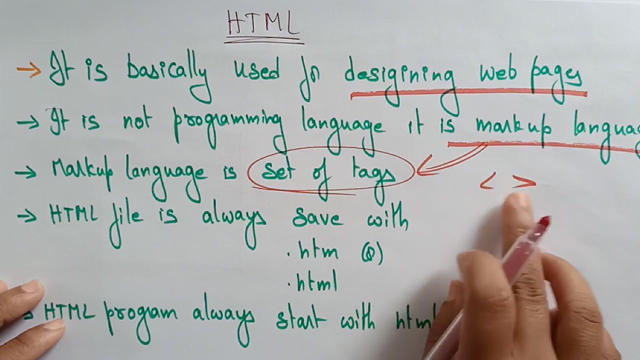 programming language. A markup language is set of tags. So here you're having the set of tags. What is the meaning of the markup language? The markup language is having set of tags. So whereas in the programming language you won't use the tags, you just write the programming code, But in the markup language you have to write everything in the form of set of tags. Tags means the open and closed brackets. So like this is a tag, The statements have to be written inside this tag. 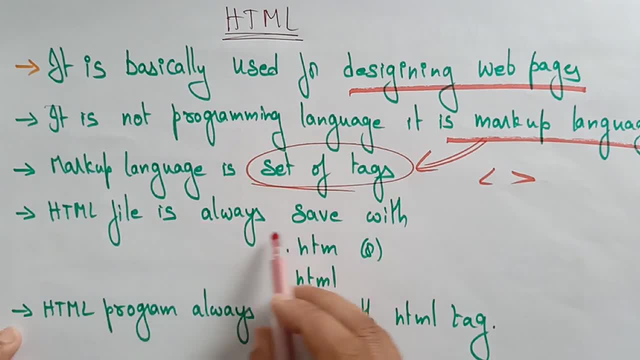 Okay, so there is a markup language. HTML files is always saves with the dot HTML or dot HTML. So you have to save the file like, suppose, a dot HTML, or you can write it as a dot HTML. So save the file with the dot HTML, then only the that file will execute in the browser. If you want to execute the files on the web browsers, you need to save it as dot HTML. Don't forget it. If it is saved in the dot document. 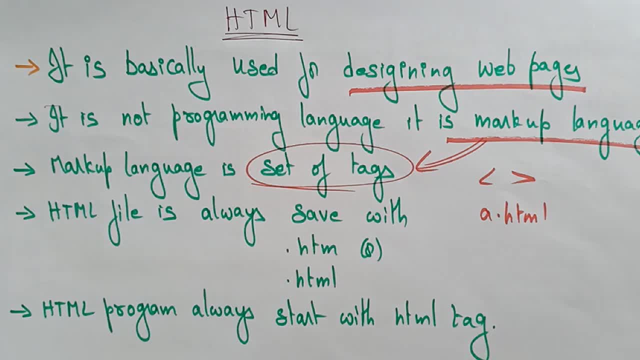 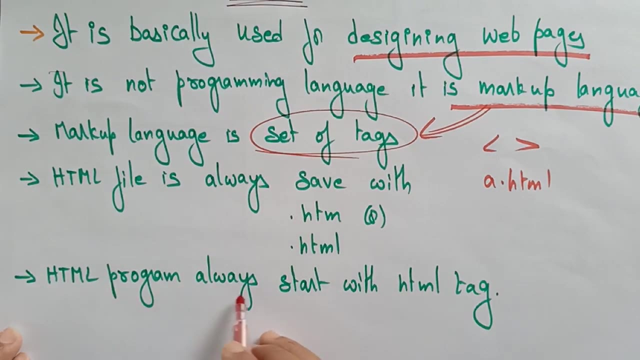 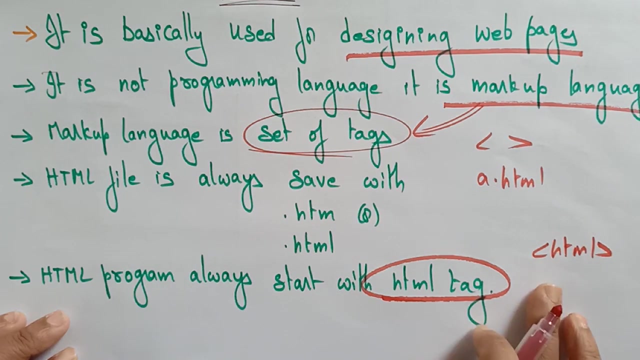 the complete the code will be appeared on the web page. If you want to show the designing part of your web page, you have to save the file as dot HTML. Okay, as it remember, so don't forget to save it as dot HTML. HTML programs always start with the HTML tag, So starts with the program as HTML tag. So this is just HTML tag. Start with the HTML tag and return everything in this here and end with the HTML tag. 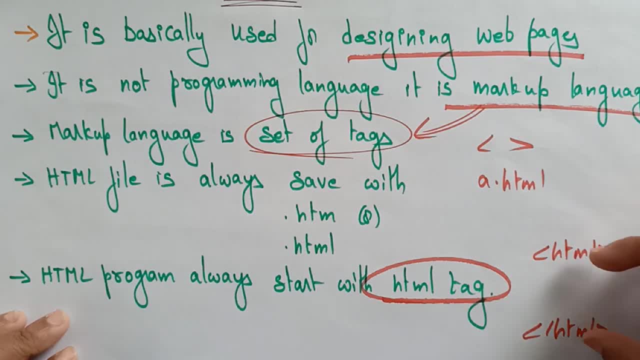 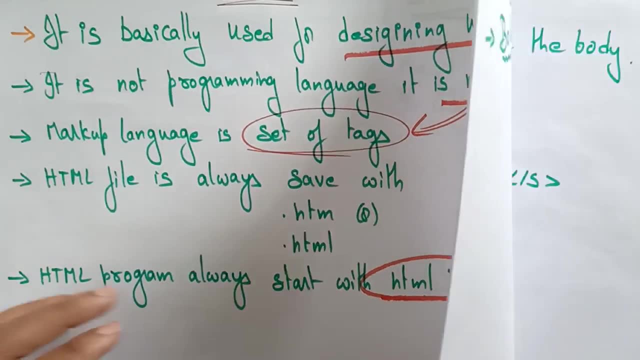 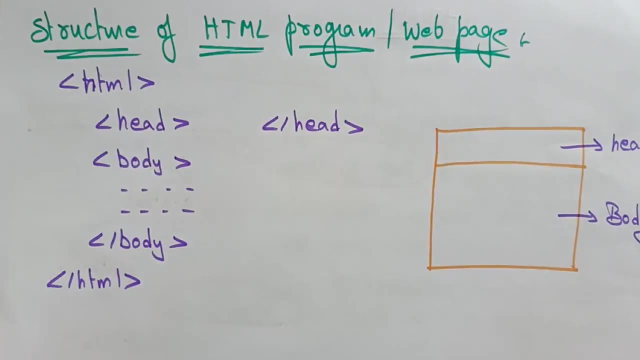 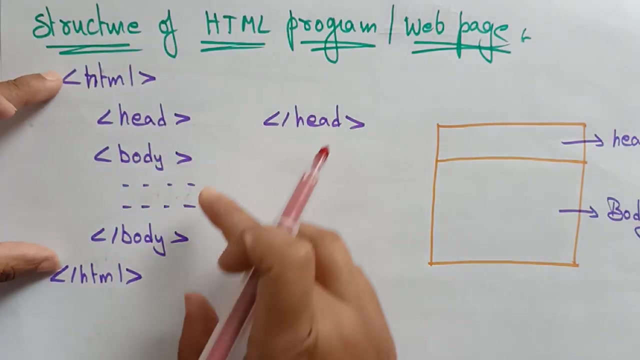 The opening and closing pack should be there. then the program will be that complete page. whatever that is present inside that will be shown on the browser. So now let's see the structure of HTML program. that is a web page, how the web page will be appeared. So the web page comes. this is the starting tag and this is the ending tag. So in between the starting tag and ending head you're having so many tags because everything I have to represent in the tag 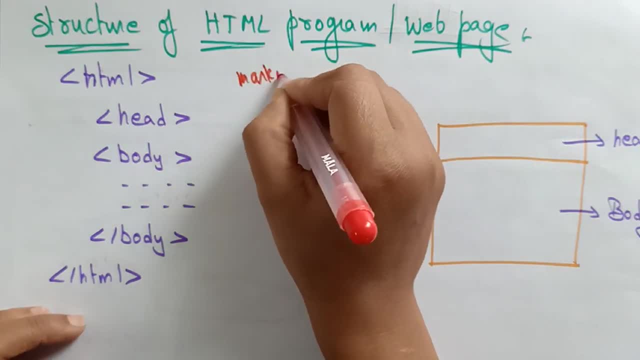 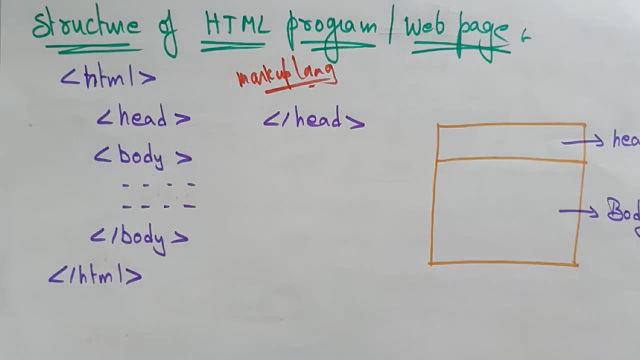 because this is a tag, representation is a markup language, So that's why we call it as a markup language, not a programming language. a markup language consisting of everything in the form of a tags. So HTML, you're having the head tag as well, as you can write here the title tag also. So in the head tag, the page that is the top most row should be the head or a title you are going to write. So this is a complete window. whatever the window that you're seeing, or 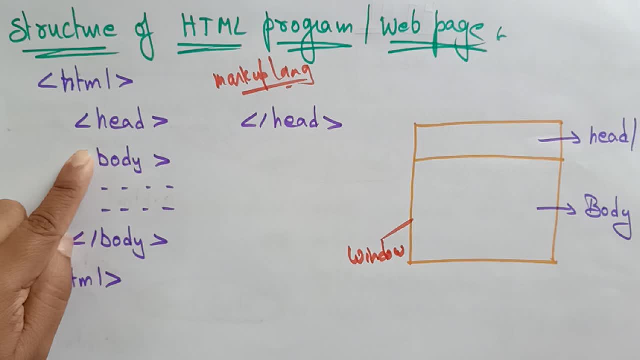 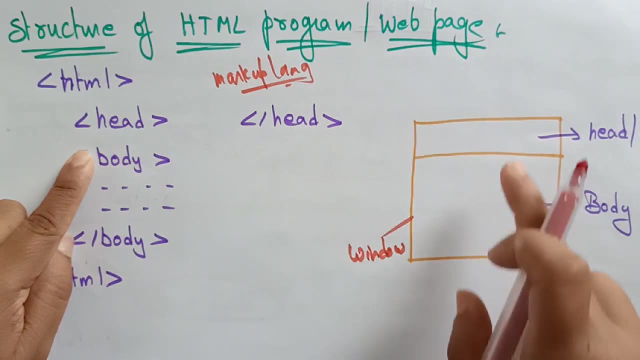 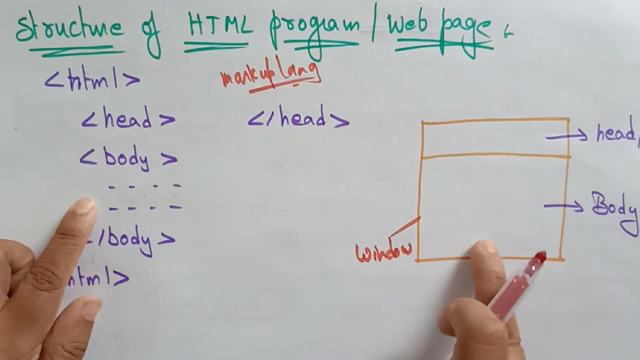 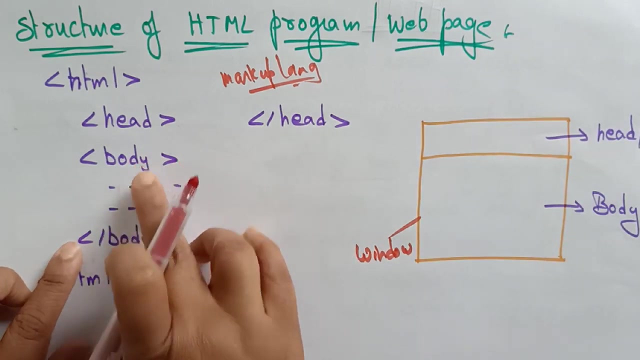 on your laptop or whatever the browser means, whatever the gadget you are open, So that is a website page, a page, that window that appear on the screen. So that screen is divided into two parts. One is the head section, the title of that page, Okay, and coming to this body section, So this part is the body section. So in this body section, whatever you want to be displayed that you have to write in between the body start tag and body end tag. So everything should be present inside. And finally, you need to 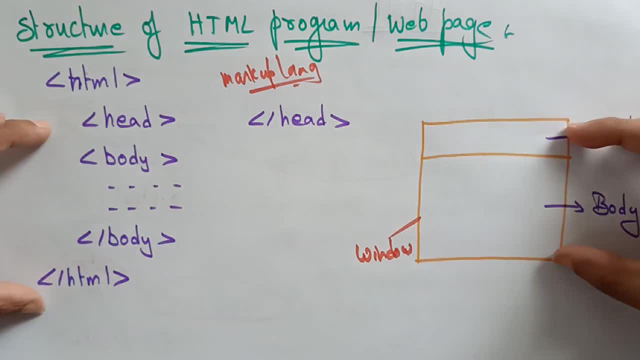 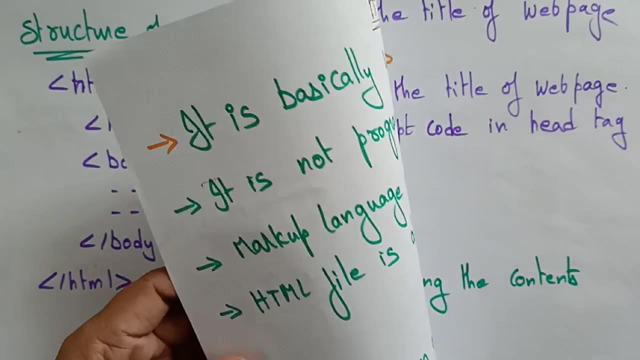 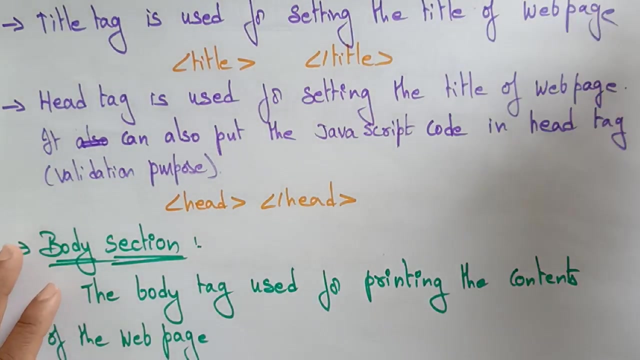 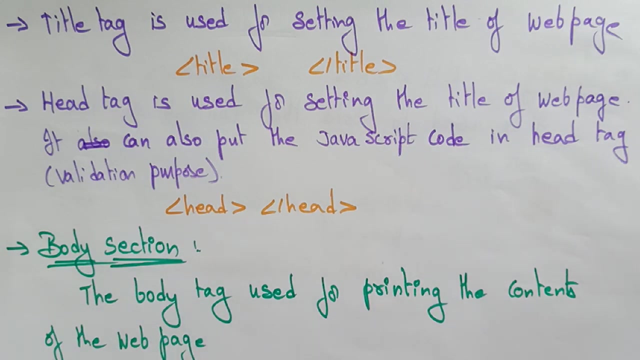 close the HTML tag. So this is just a: creates a page with two rows. Okay, this is a structure of HTML program or a web page. So the title tag- whatever you are seeing here, the head or the title tag- is used for setting the title of the web page. So what title of the web page that you want that you can write here: Okay, that is the main heading of the here, like something: like: you want to create education for you. Okay, it's.